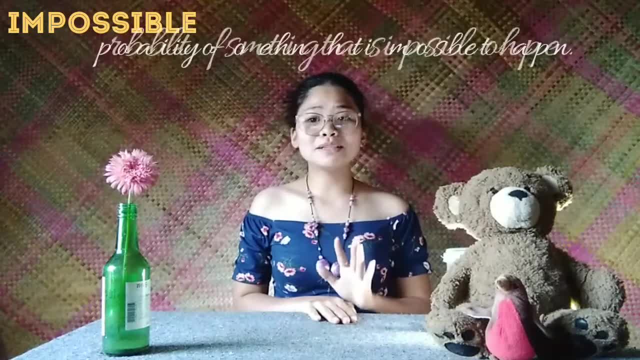 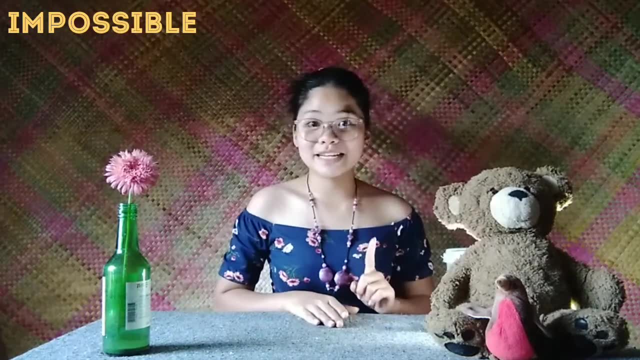 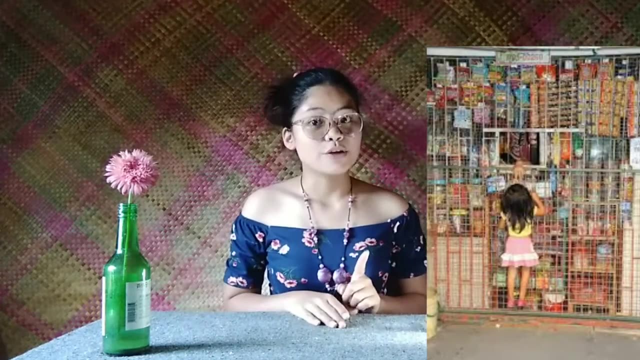 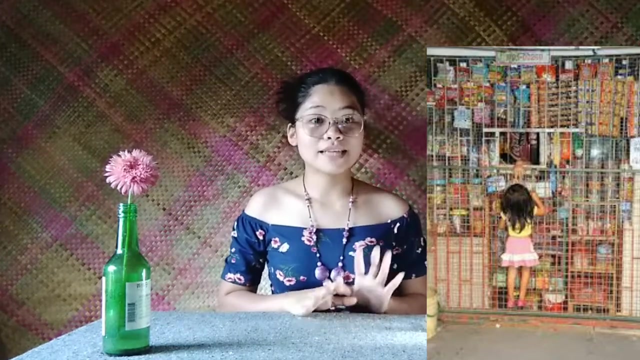 term is the impossible or the probability of something that is very impossible to happen. Take this as an example. A little girl buys a candy in the store. The saleslady gave her the chance to pick a candy. in a bottle There are ten lollipops, five kindermen. 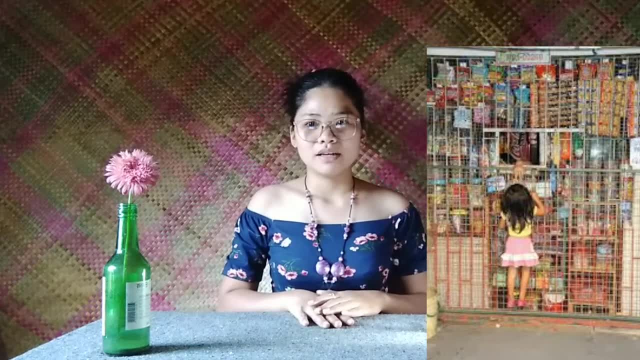 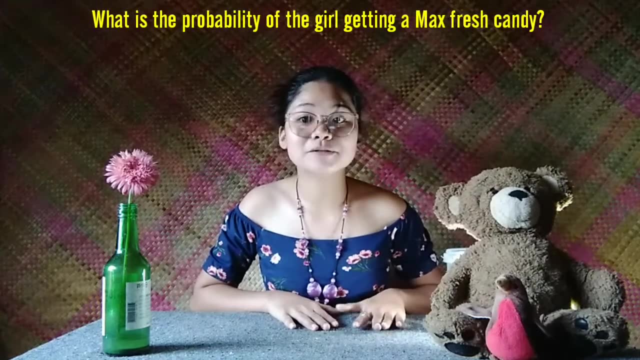 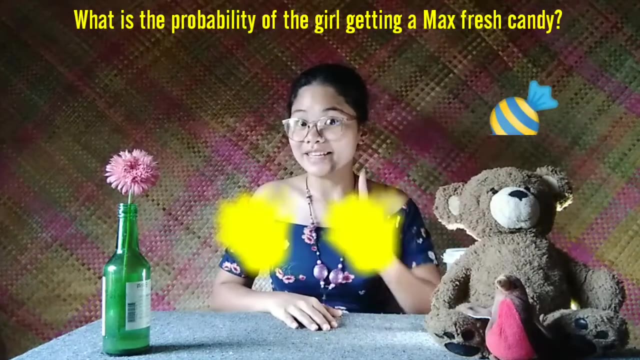 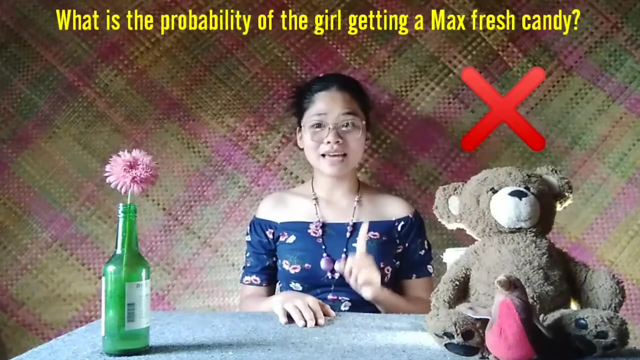 and one white rabbit inside. And the question is: what is the probability of the girl getting a max fresh candy? What do you think? I think nothing. Yes, you think it right. It's nothing Or impossible. Did he get a max fresh candy? Yes, there are many candies inside the bottle. 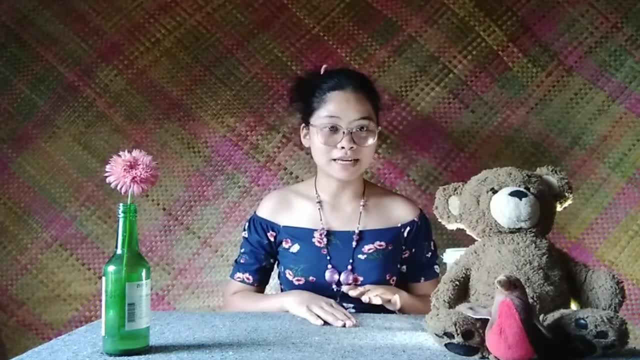 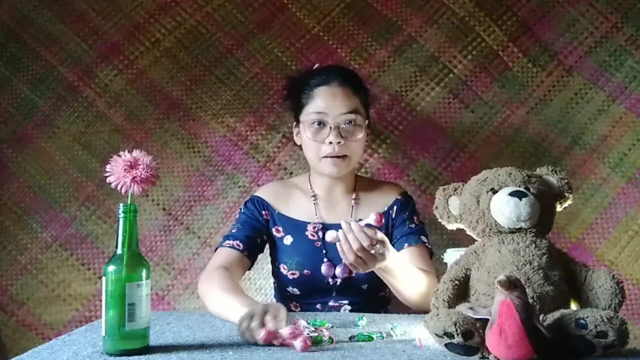 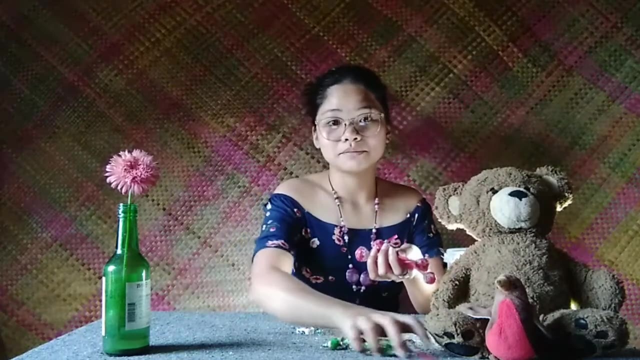 but nothing is a max fresh candy inside. Look at this example. So I have here ten lollipops, Ten lollipops and five kindermen and one white rabbit. So let's see What is the probability of the girl getting a max fresh candy. What is the probability of the girl getting a max? 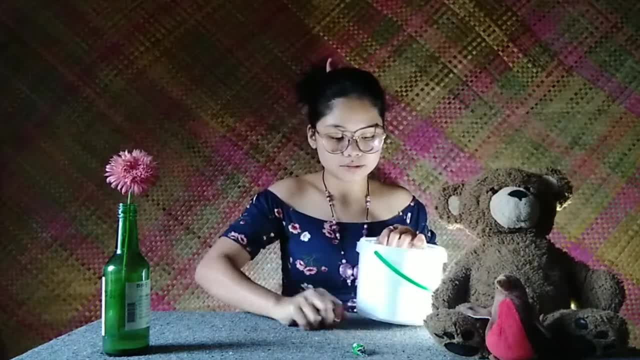 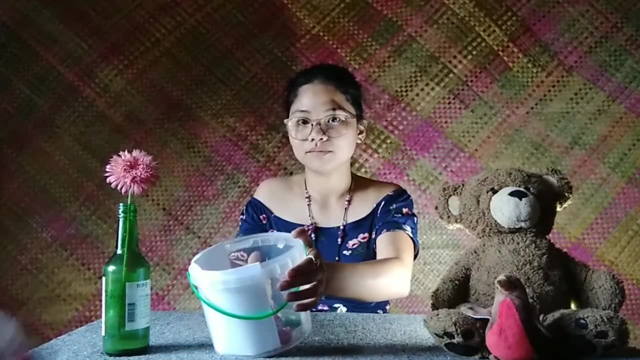 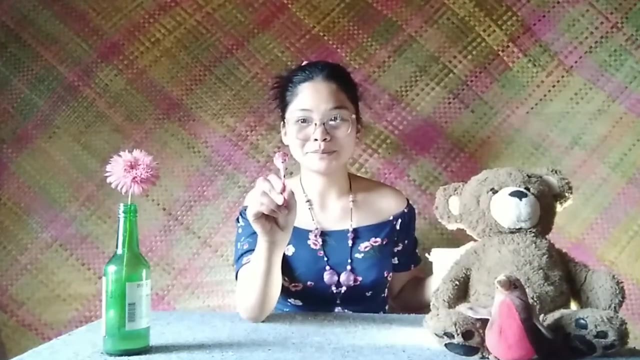 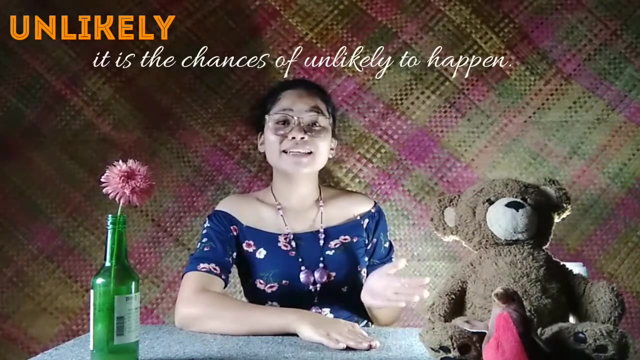 fresh candy. So let's put it in the box or in the bottle. So let him pick. What did he pick? One lollipop, So he picked one lollipop. Second term is unlikely. It is where the chances are unlikely to happen. Take this as an example. 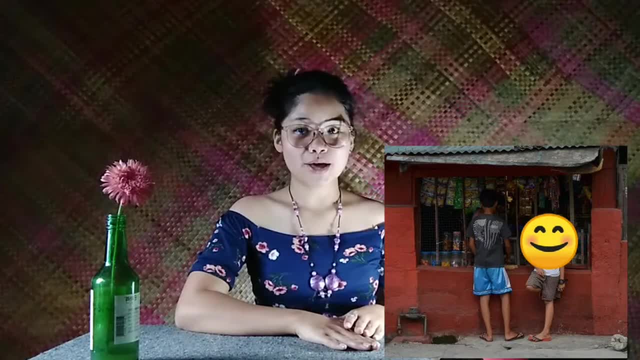 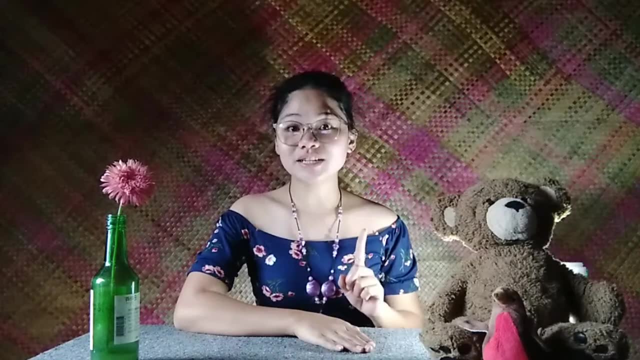 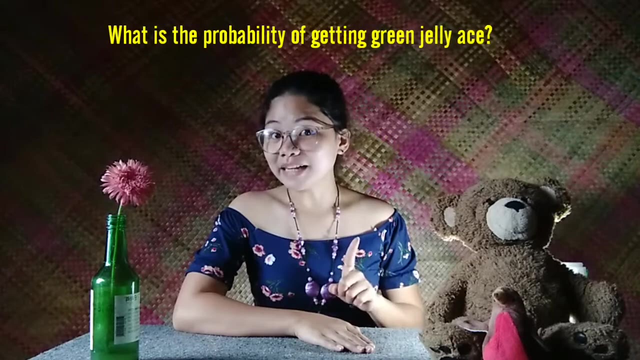 Jake buys a lollipop in the store. There are five yellow lollipops and one green lollipop, So there are six in all, And the question is: what is the probability that Jake is getting a green lollipop? So 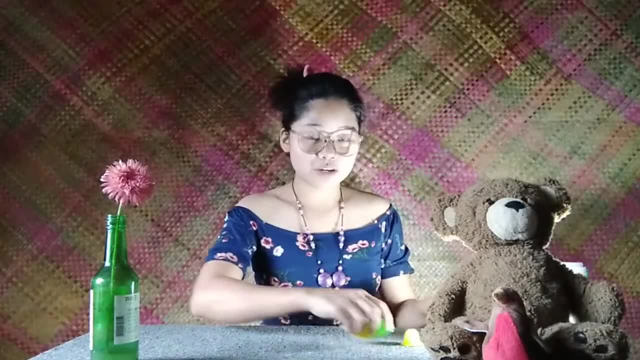 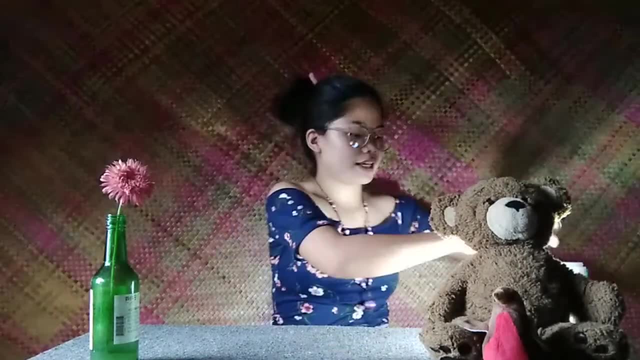 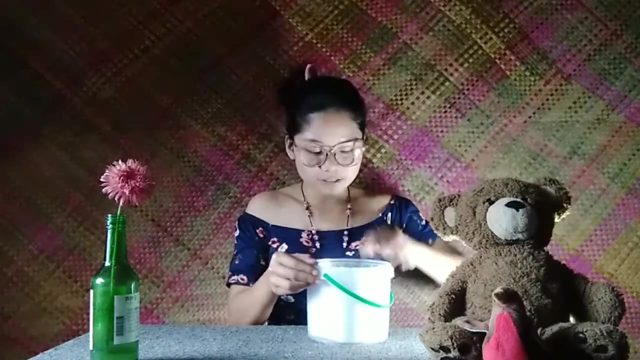 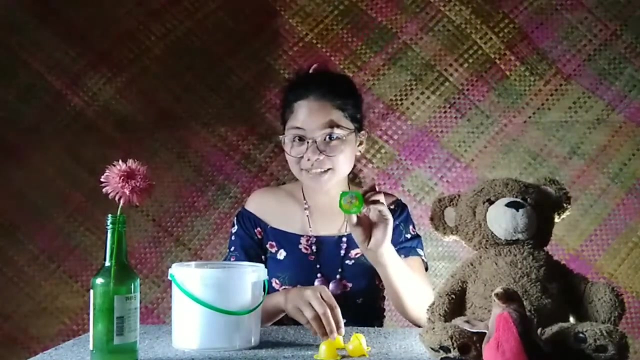 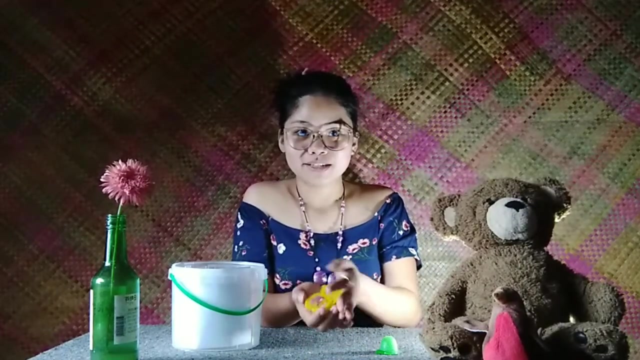 take a look. I have here a lollipop, one green, five yellow lollipop. So we put it in the bottle, So we let him pick. So let's try to look at it again. Green lollipop is still here and there are four yellow lollipops left. So Jake picked a yellow. 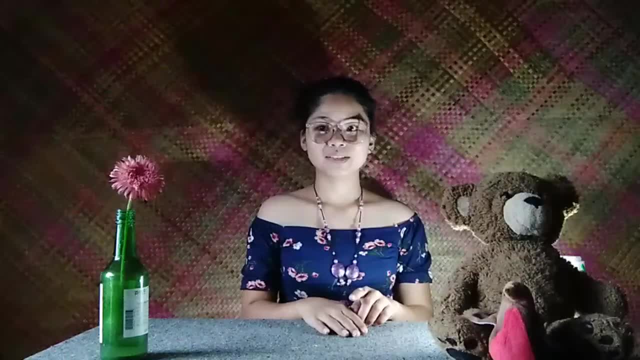 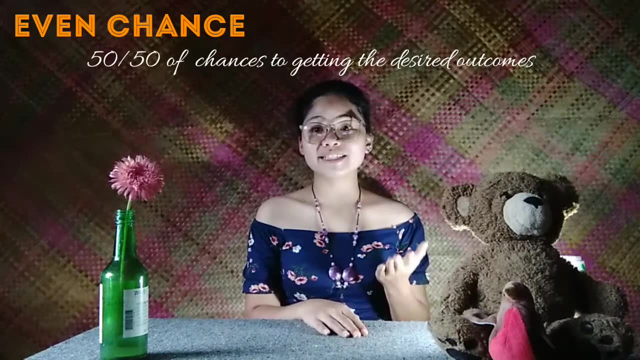 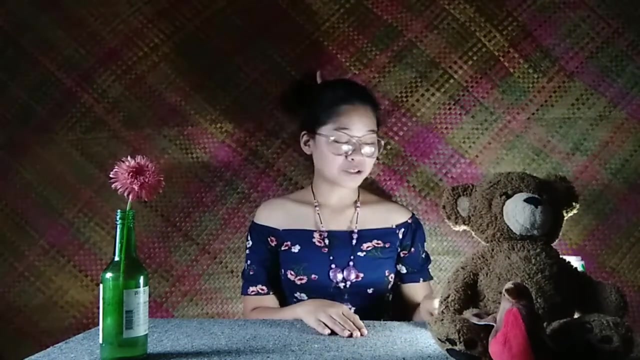 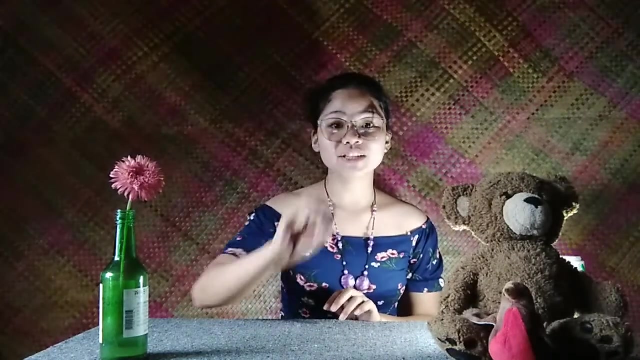 lollipop. Okay, Got it. The third term is the even chance. It is 50-50 chances of getting the desired outcome. For example, I chose a coin. This is one piece of coin And the question is: what is the probability? 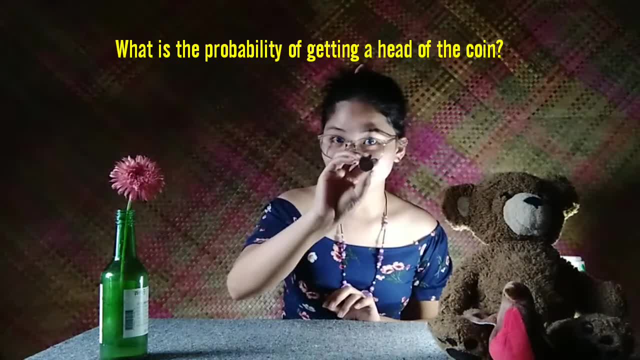 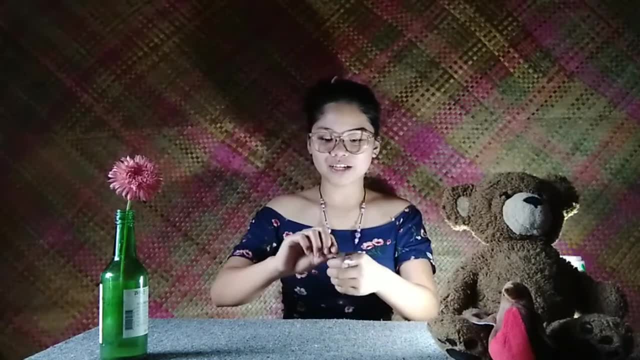 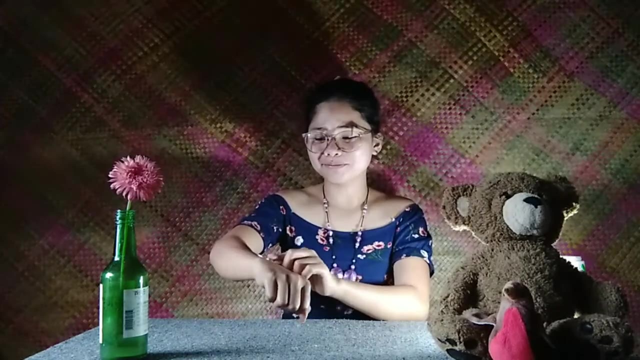 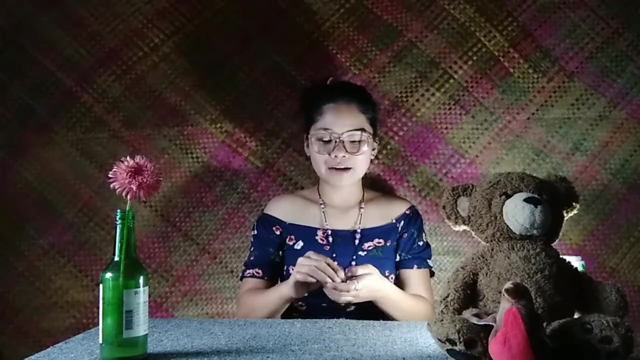 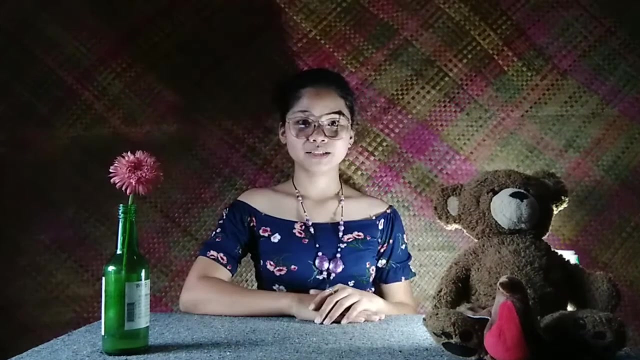 that I got the head of Ed. Oh, get the head. let's have a try. oh sorry, one more time again. oh no, it's a tail, let me have one. yes, success, it is a hit. the fourth term is likely. it is more than 50, 50 of. 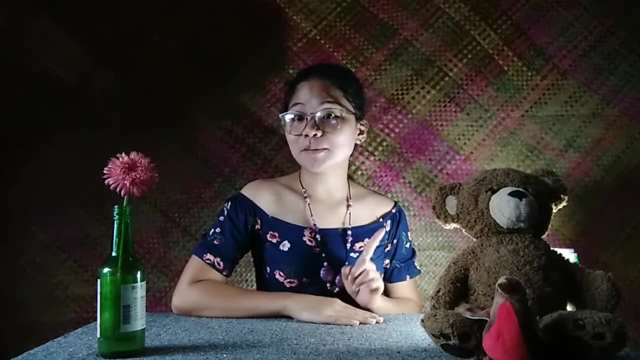 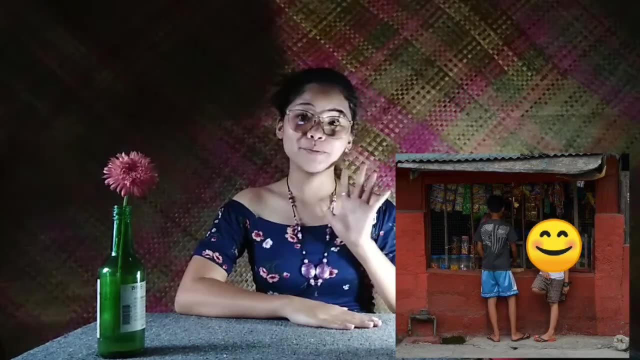 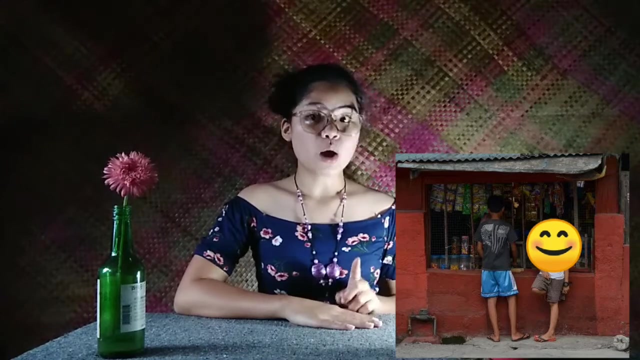 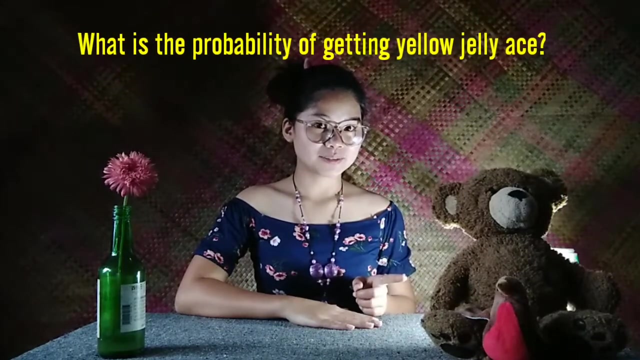 chances. let's have the same example of unlikely term. Jake buys a jelly ace in the store. there are five yellow jellies and one green jelly ace, so there are six in all, and the question is: what is the probability that Jake getting a yellow jelly ace? you can have your guess. 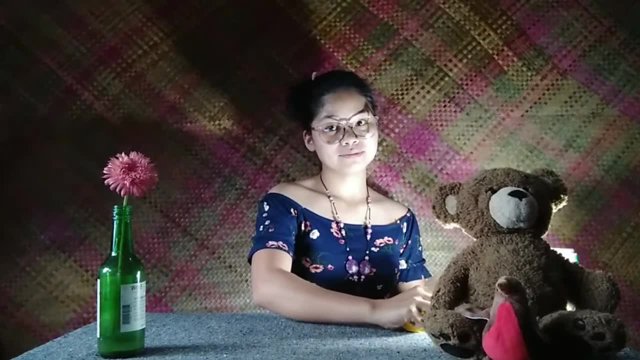 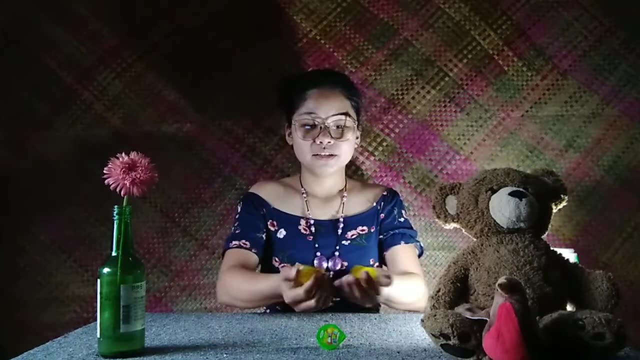 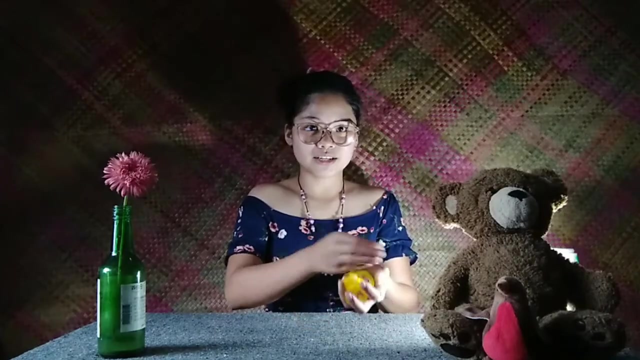 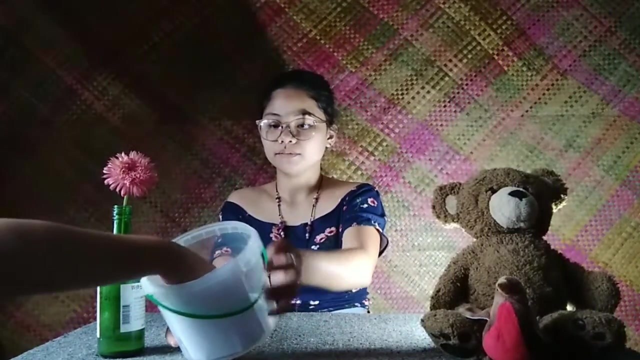 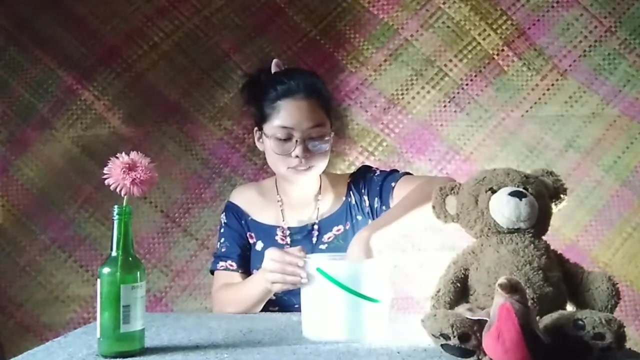 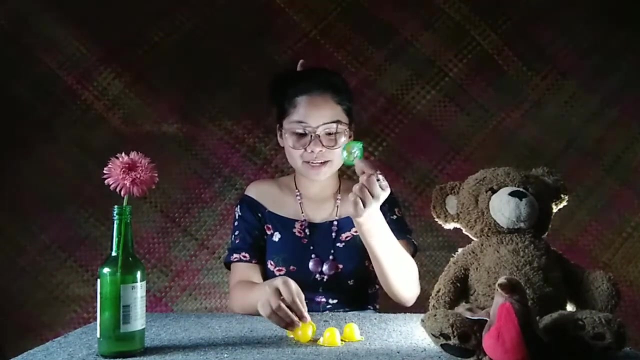 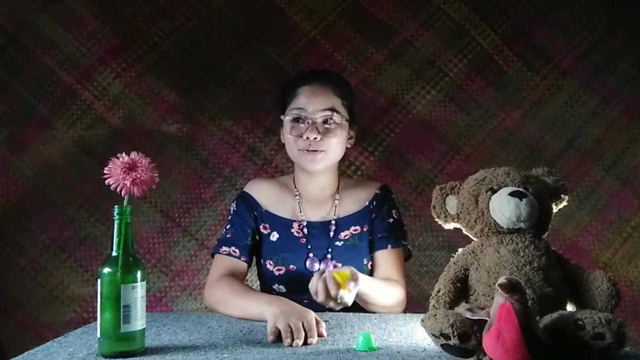 now, I guess the chances is five, six. so let's have a try. I have here five yellow jelly ace and one green jelly ace, so let's see you. let's take a look. what is the missing one? so the green is here and the yellow. there are four yellow, so that this is a missing one. so, Jake, pick a yellow jelly. 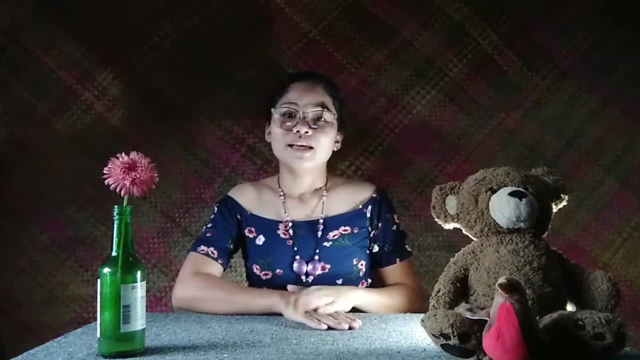 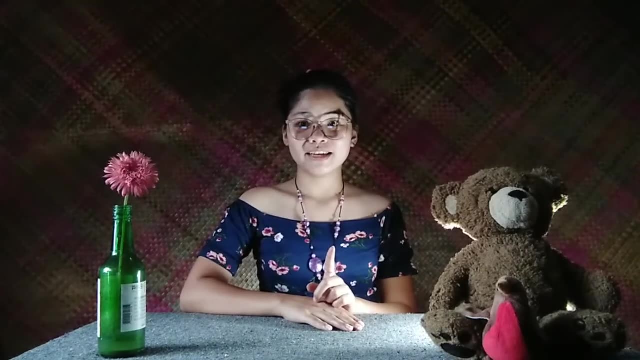 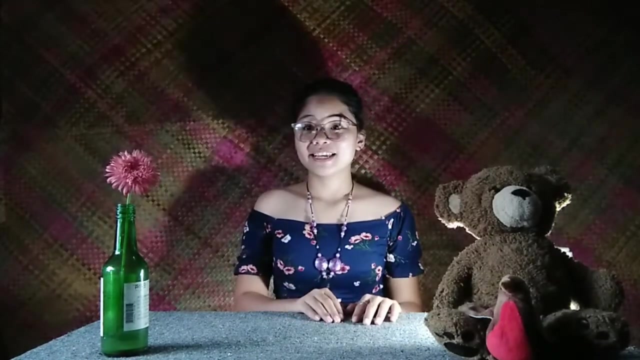 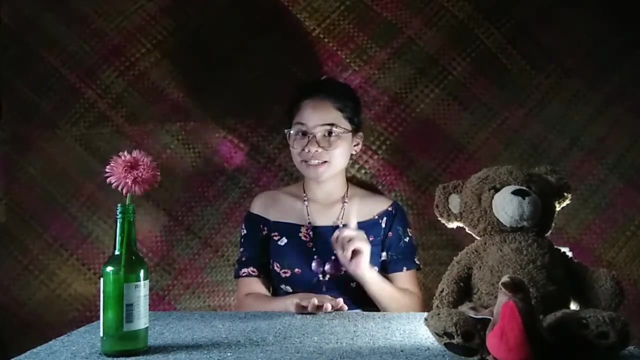 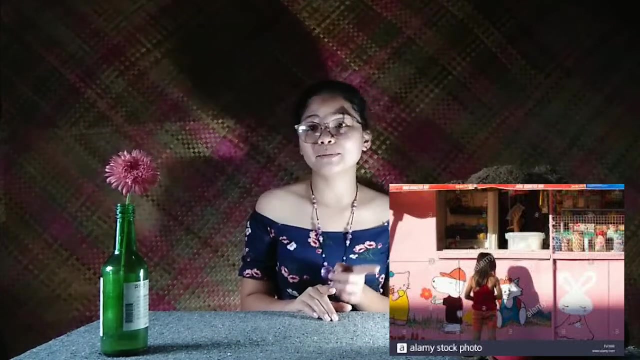 ace, and you're right. he picked the yellow jelly ace for it is very likely a chance because there are too many. the last term is external. it is a one hundred percent of probability. take this an example: shire wants you drink a soft drink. she went into the store and avellma sell only royals of drinks like. 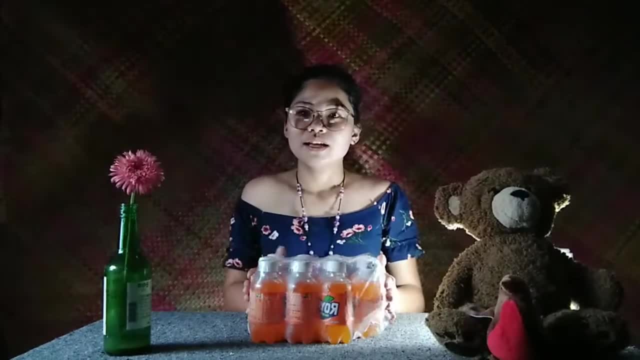 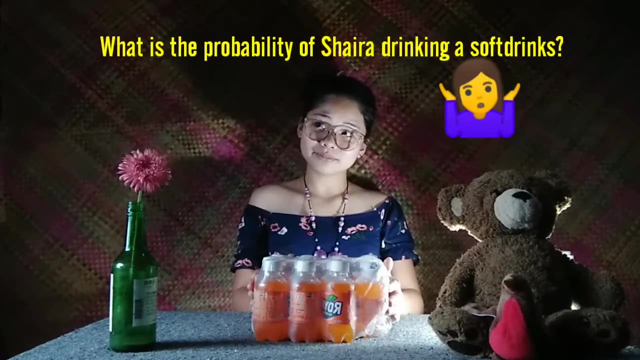 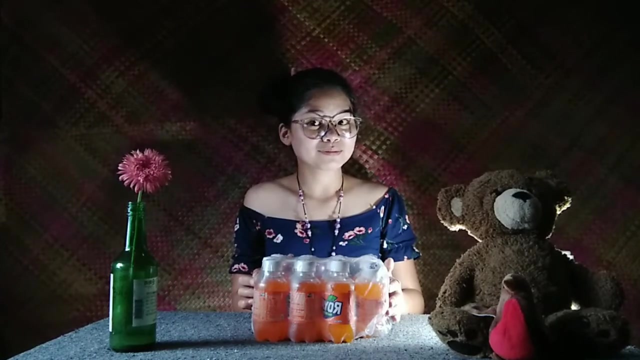 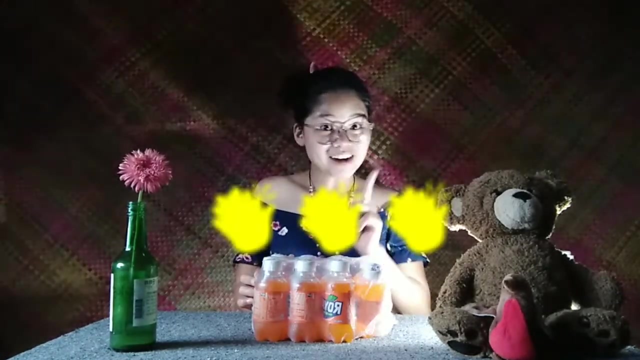 like this. So what is the probability that Shira drinks is soft drinks? Of course, a certain. Why do you say so Really? is the soft drink and Shira doesn't specified any flavor? as long as it is soft drink, Very good. Shira doesn't specified any flavor, as long as it is soft. 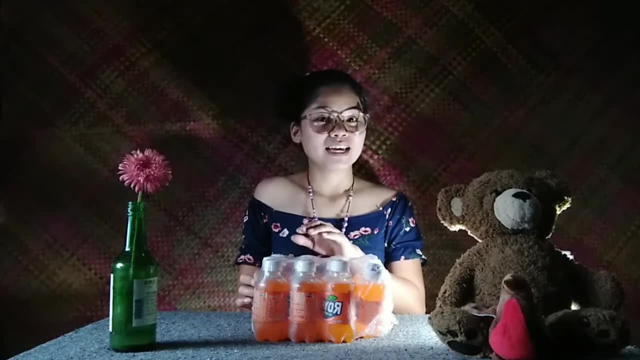 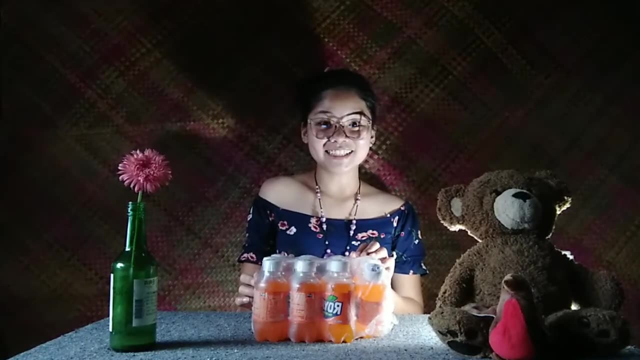 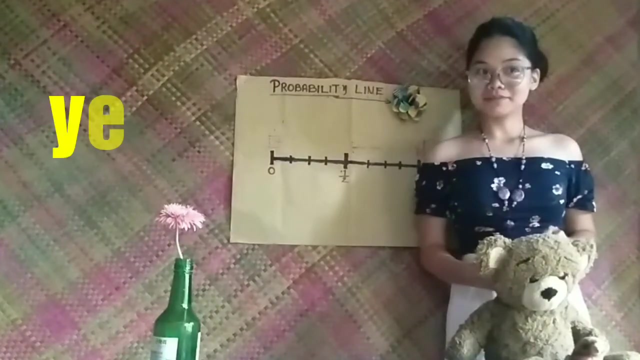 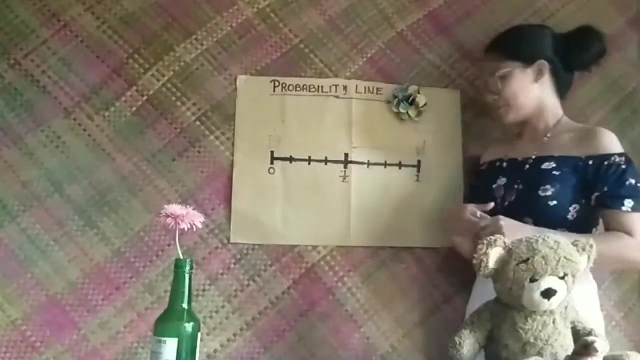 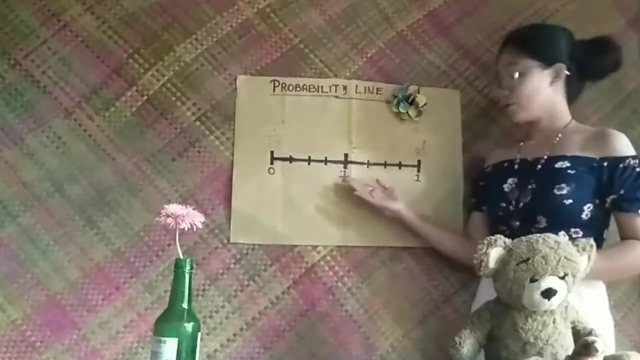 drinks, and royal is a soft drink, so it is certain that he drink a one. royal Got it, Yes. Now do you know that probability can be a fraction too Good, Now I'll show you the probability line, This one: It starts with zero, one half at the middle and one at the end.